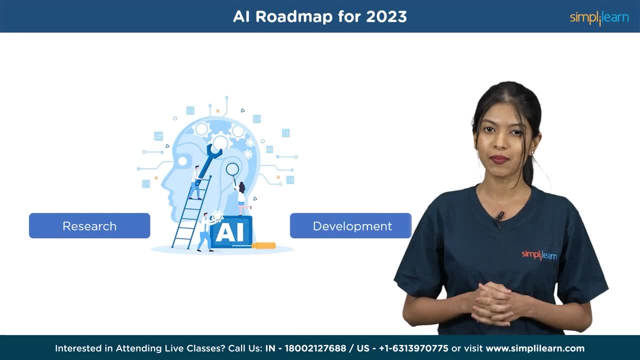 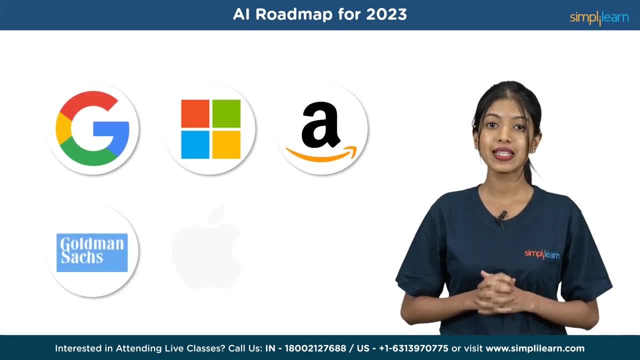 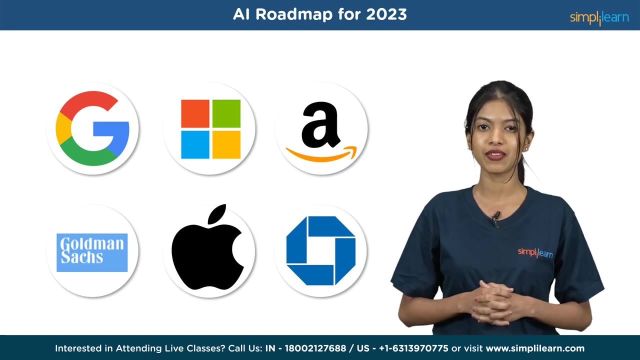 skilled AI engineers to contribute to their research, development and implementations of AI technology. Among these top companies are Google, Microsoft, Amazon, Goldman Sachs, Apple and JPMorgan Chase. Therefore, top companies hiring AI engineers provide excellent opportunities for aspiring. 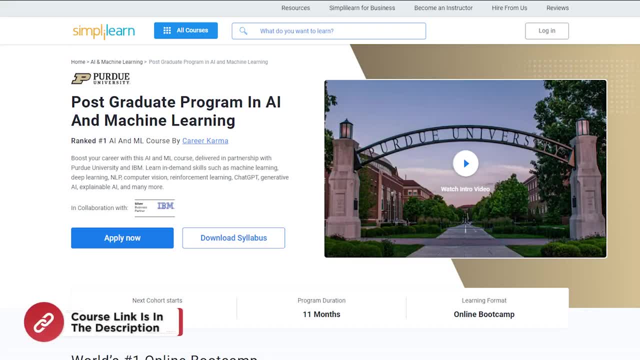 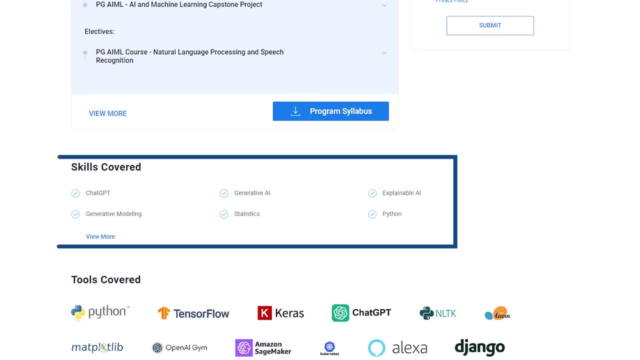 professionals. On that note, elevate your career with our AI and ML course, developed in partnership with Purdue University and IBM. Gain expertise in high-demand skills such as machine learning, deep learning, NLP, computer vision, reinforcement learning, chat, GPT. 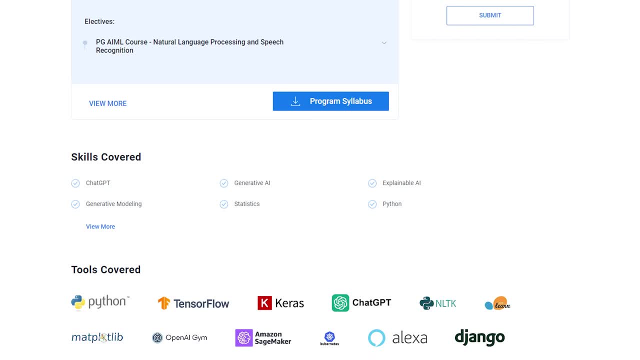 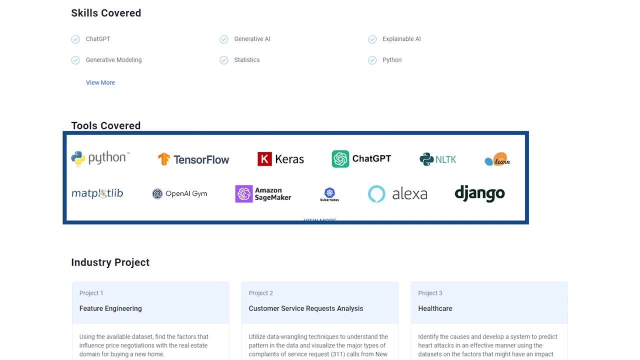 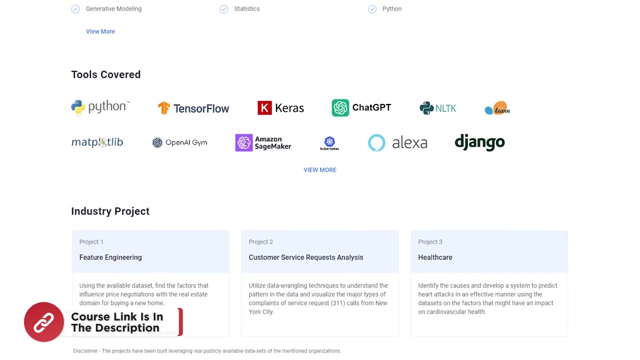 generative AI and more. Unleash your potential and unlock exciting opportunities in the world of AI and ML. This course covers tools like Python, TensorFlow, Keras, ChatGPT, OpenAI, GIMP, Matplotlib and many more, So hurry up and find the course link in the description box for more details. Our learners- 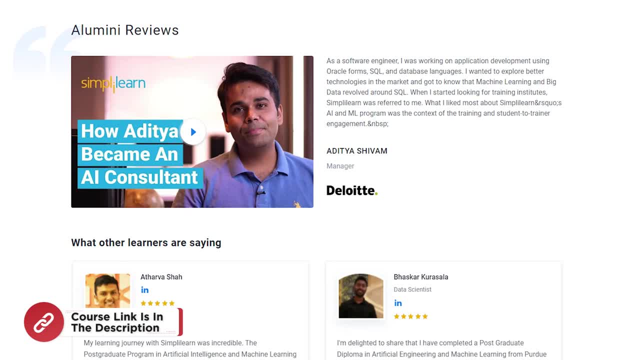 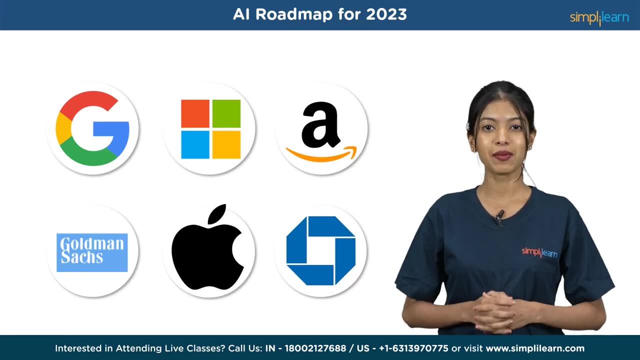 have experienced huge success in their careers. Listen to their experience. Find the SimplyLearn course review link in the description box. Without any further delay, let's dive into the topic now. If you decide to become an AI engineer, what are some of the steps you can follow to achieve your goal? 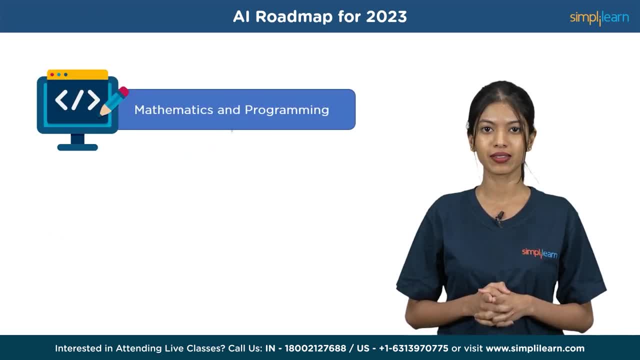 Firstly, obtain a strong foundation in mathematics and programming. Gain a strong foundation in creating mathematical concepts like linear algebra, calculus and probability theory. In addition to that, it's crucial to acquire mastery of programming languages like Python, commonly used in AI, and become proficient in coding. 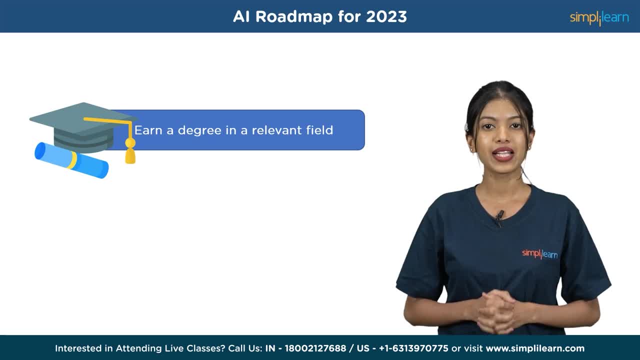 Then earn a degree in a relevant field. That means earn a bachelor's or master's degree in computer science, data science, AI or a related field to gain a comprehensive understanding of AI principles and techniques. Next, gain knowledge in machine learning and deep learning. 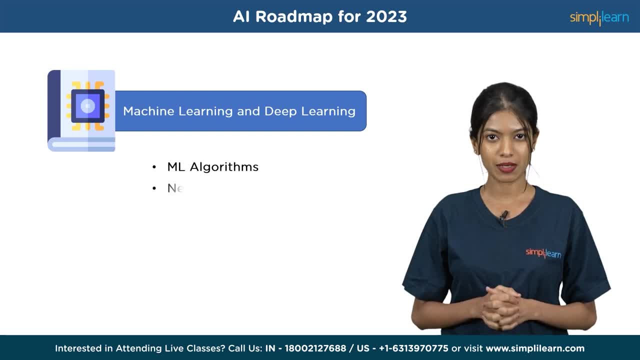 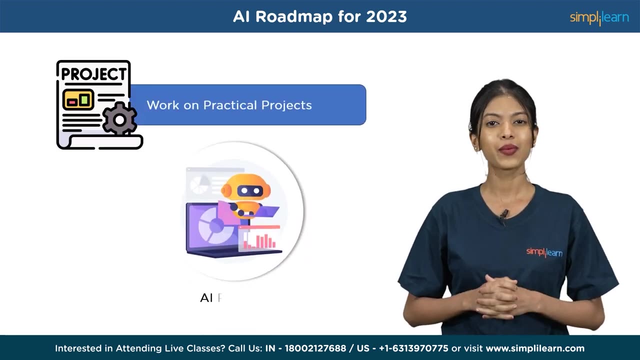 To become an AI engineer, develop familiarity with ML algorithms, neural networks and deep learning frameworks- example: TensorFlow, PyTorch- to train and optimize models using real-world dataset, Followed by that work on practical projects. Gain hands-on experience and showcase your skills by working on AI projects. 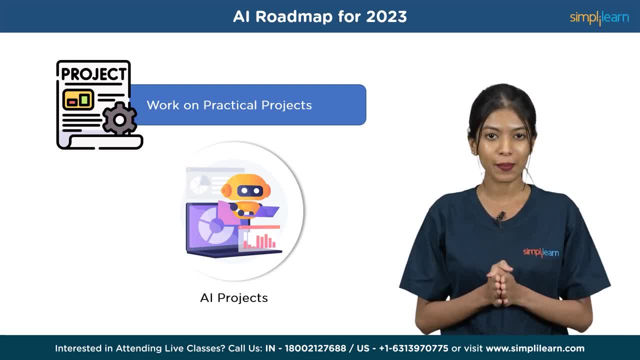 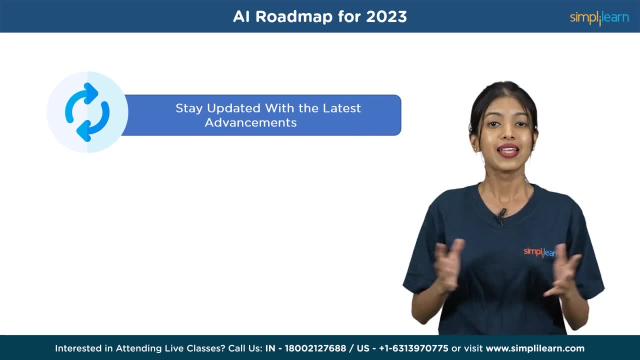 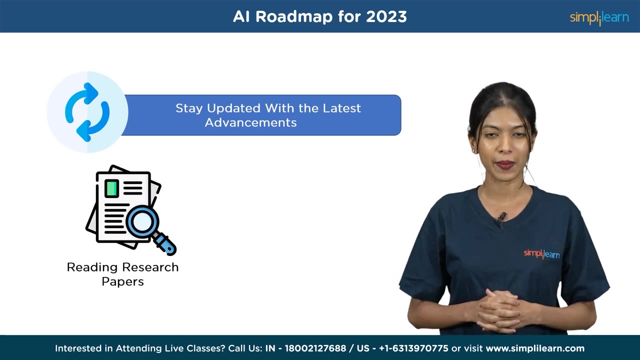 Moreover, build a portfolio of projects demonstrating your ability to solve AI problems, impressing potential employers. Then stay updated with the latest advancements. Stay updated with the latest trends and research in AI, a rapidly evolving field, and expanding your knowledge by reading research papers. 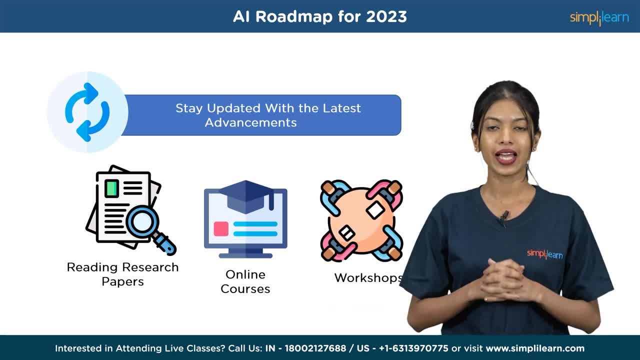 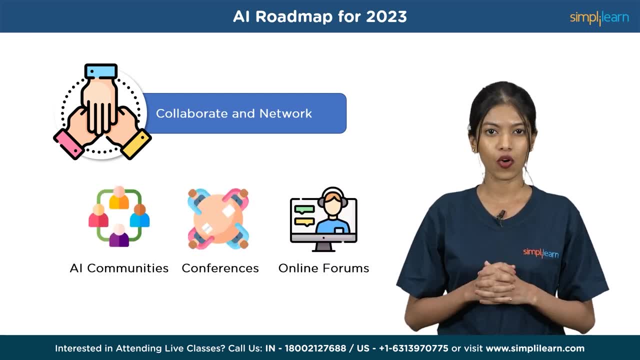 participating in online courses and workshops and joining AI communities. Next, collaborate and network. Engage with AI communities, attend conferences, participate in online forums and connect with professionals in this field. Collaborating with others can enhance your learning experience and open new opportunities. 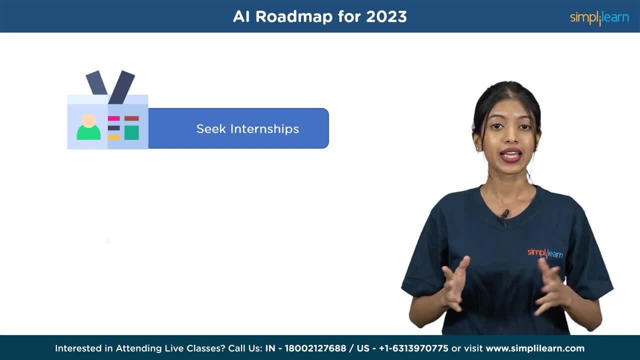 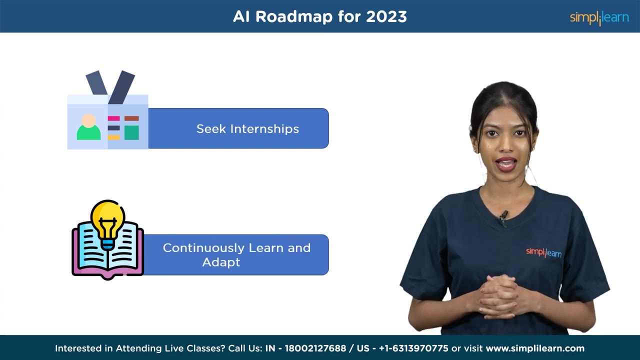 Later seek internships or entry-level positions. Gain practical experience through AI internships or entry-level roles in industry or research institutions. This provides valuable exposures and helps develop your skills. Finally, continuously learn and adapt In the rapidly evolving field of AI. stay updated on new developments. 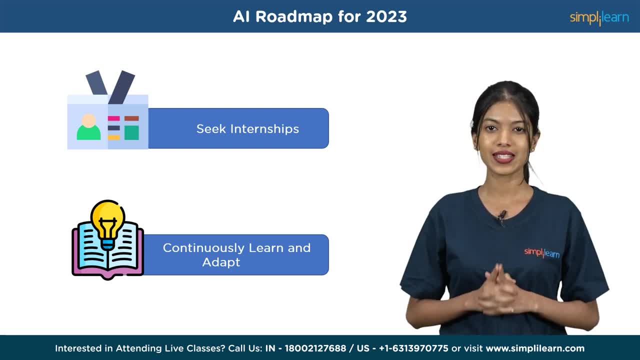 explore specialized areas and embrace emerging technologies and technologies. Learn more about AI technology and tools to pursue a career as an AI engineer. Now that we have covered the essential steps to become an AI engineer, let's explore the necessary programming languages and algorithms for aspiring AI engineers. 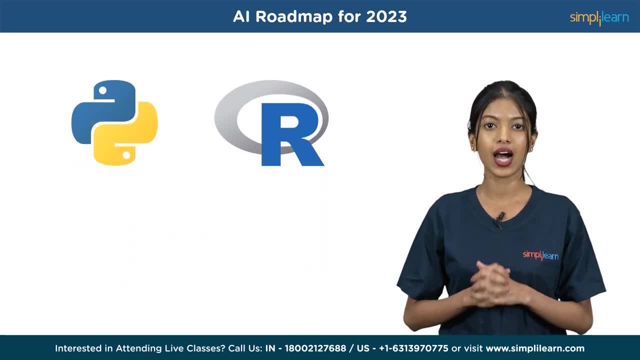 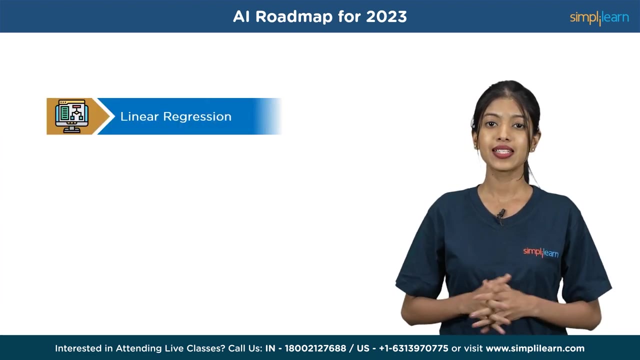 So mastering programming languages like Python, R, Java and C++ is vital for acquiring proficiency in AI. These languages enable you to construct and deploy models effectively. Additionally, it would help if you gain a thorough understanding of machine learning algorithms such as linear regressions, k-nearest neighbors, name base and support vector machines. 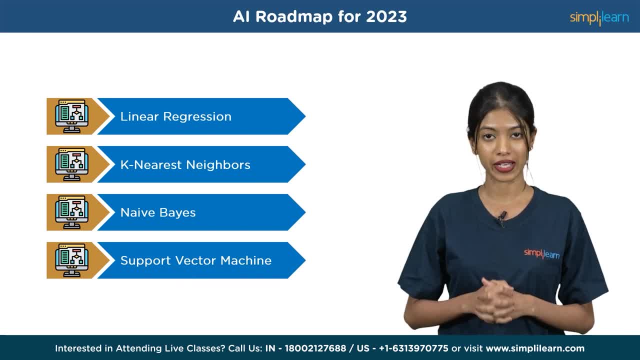 These languages and algorithms are fundamental tools in the field of AI. They will enable you to develop and implement effective artificial intelligence models. Now let's take a minute to hear from our learners who have experienced huge success in their career. You need to keep updating your skills. 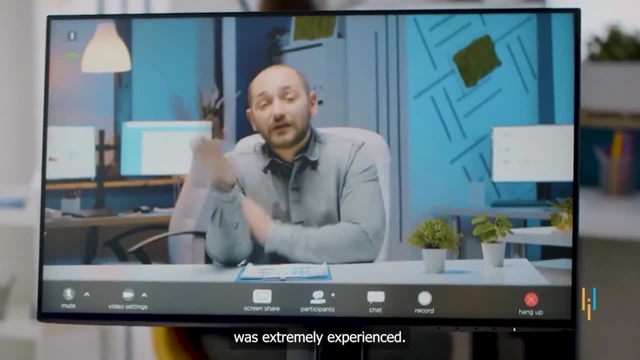 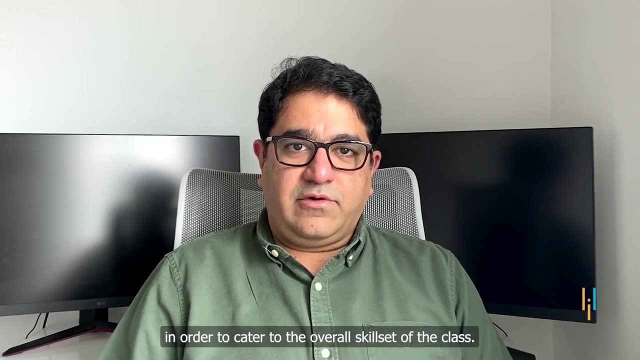 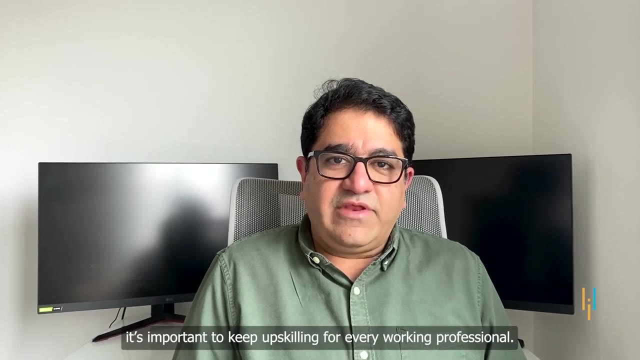 The course material was comprehensive and the faculty was extremely experienced. The faculty was able to adjust Their teaching style in order to cater to the overall skill set of the class. In the rapidly evolving world of technology, it's important to keep upskilling for every 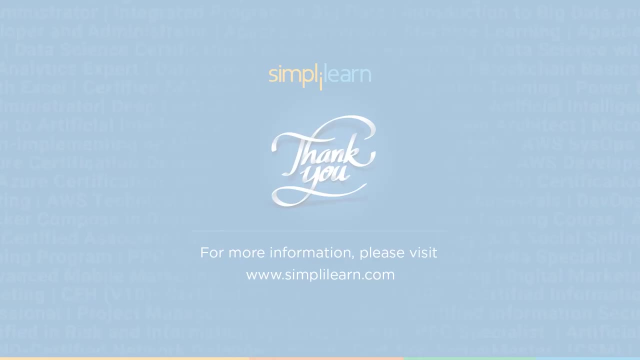 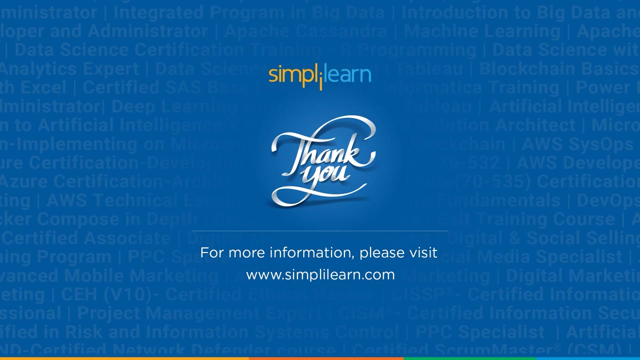 working professional, Stay relevant, Continue learning. With this, we have come to the end of this Artificial Intelligence Roadmap in 2023.. I hope this video was informative and interesting. If you have any queries regarding topics covered in this video or need help opting for this, 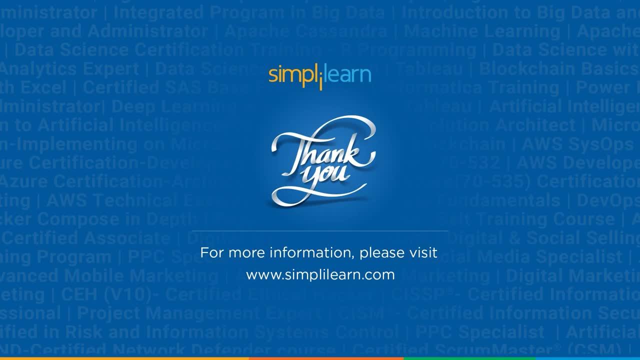 course. please let us know in the comment section below. Our team of experts will happily resolve all your queries. Thank you for watching. Until next time, stay safe and keep learning.